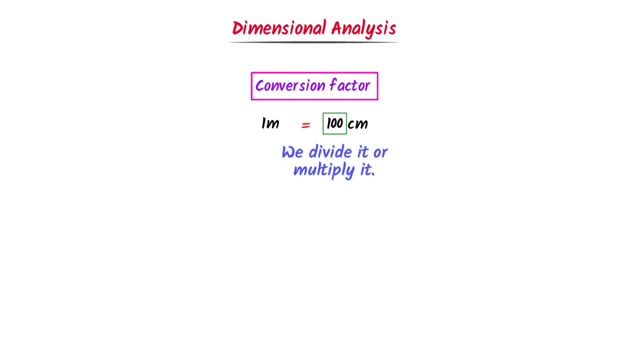 if we convert meter to centimeter, we have to multiply or divide by this conversion factor. Similarly, we know that one kg is equal to thousand grams. Here the conversion factor is thousand between kg and grams. Hence note it down that conversion factor is a number used to convert. 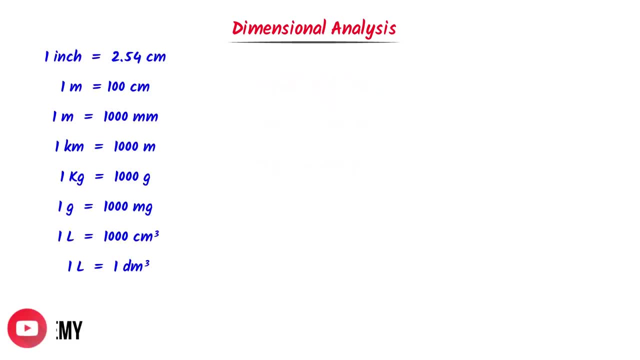 units. Now consider this list of some basic units. Remember that at the left side these are bigger units, while at the right side these are smaller units. Now my personal trick is BS. I mean bigger and smaller. If I go from a bigger unit towards a 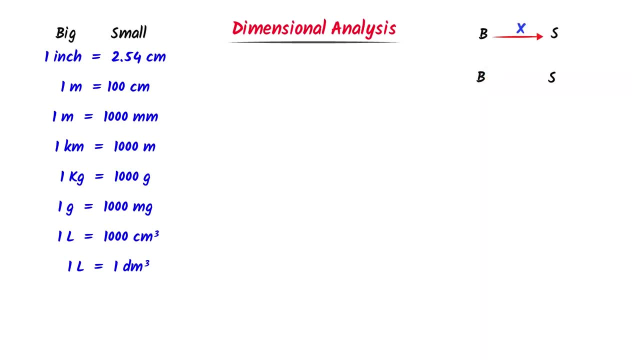 smaller unit, I multiply it by the conversion factor. Secondly, if I go from a smaller unit towards a bigger unit, I divide it by the conversion factor. For example, convert 50 inch to centimeter. We know that inch is a bigger unit and centimeter is a smaller unit. 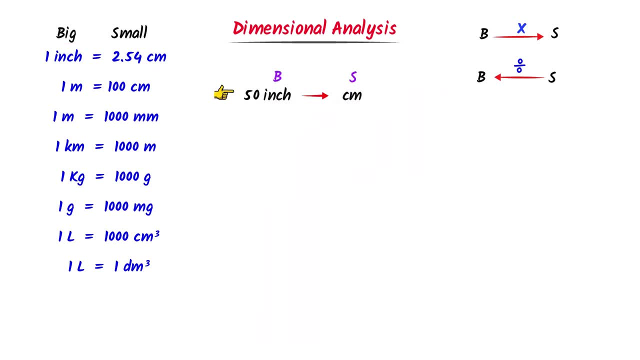 I write bigger and smaller. Here I go from bigger to a smaller unit. I will multiply 50 by conversion factor. Here the conversion factor between inch and and centimeter is 2.54.. After calculation I get 127 centimeter. Secondly, convert 50 centimeter. 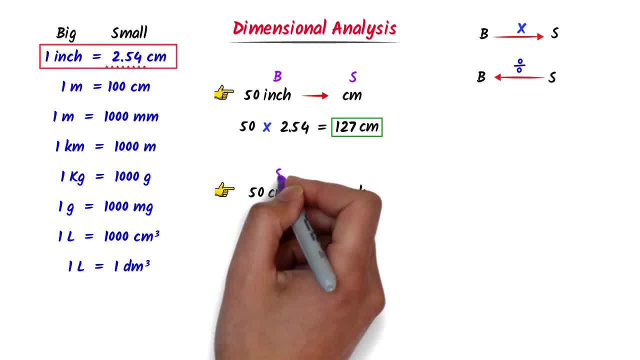 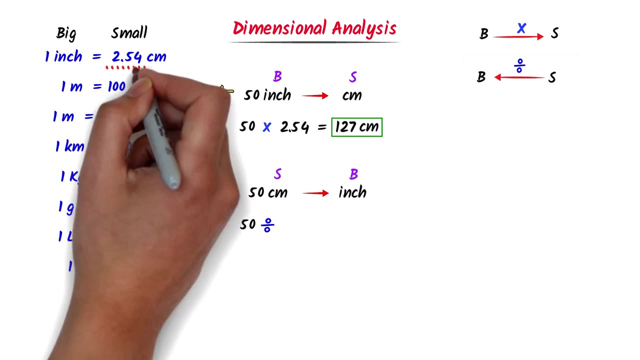 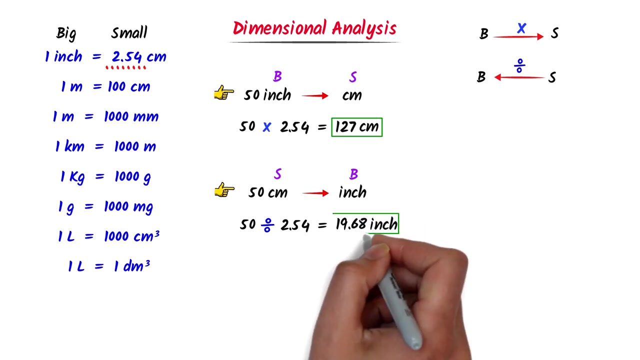 to inch. We know that centimeter is a smaller unit and inch is a bigger unit. Here I go from a smaller to a bigger unit. I will divide 50 by the conversion factor. We can see that the conversion factor is 2.54.. After calculation I get 19.68 inch. So using this simple method, 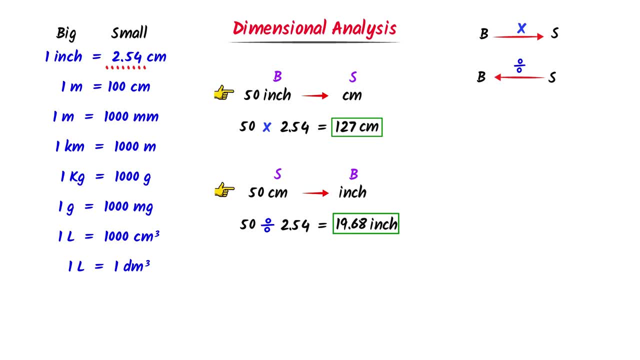 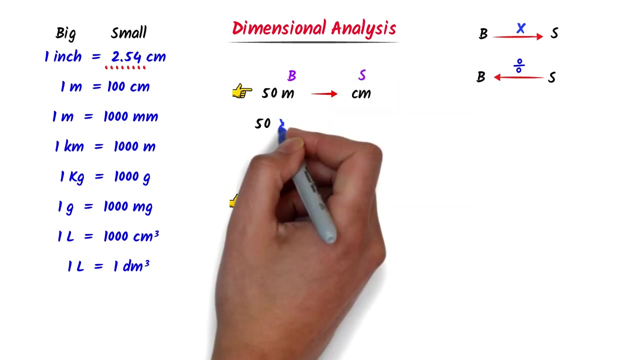 I can easily convert one set of units to another set of units. Now consider this question: Convert 50 meter to centimeter and 200 centimeter to meter. Pause the video and try to solve them. Well, I run Now. meter is bigger unit and centimeter is smaller unit, So I multiply it by the conversion. 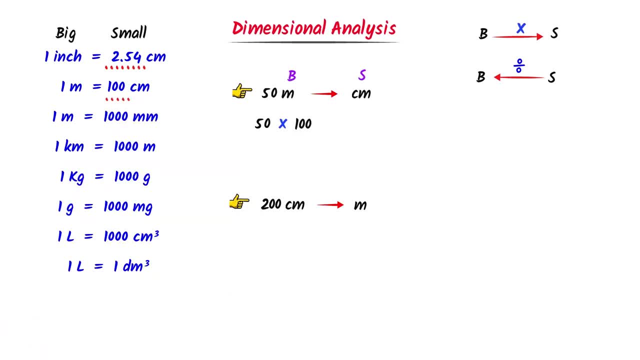 factor, which is 100.. After calculation, I get 5000 centimeter. Secondly, I write 200.. Now, centimeter is a smaller unit and meter is a bigger unit. So I divide it by the conversion factor, which is 100.. 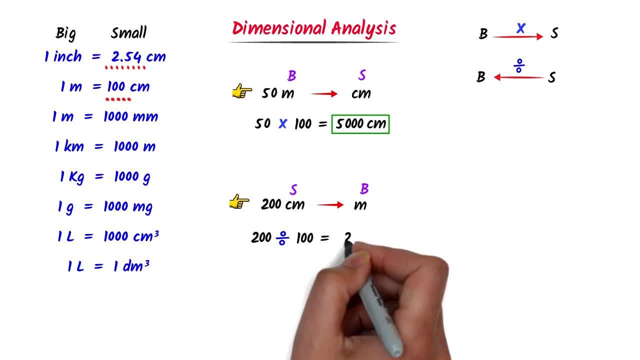 After calculation I get 2 meter. So these are the answers of these two questions. Now let me teach you some medium level questions. Convert 8000 millimeter to kilometer. We know that there is this relationship between meter and millimeter, while there is also this relationship between 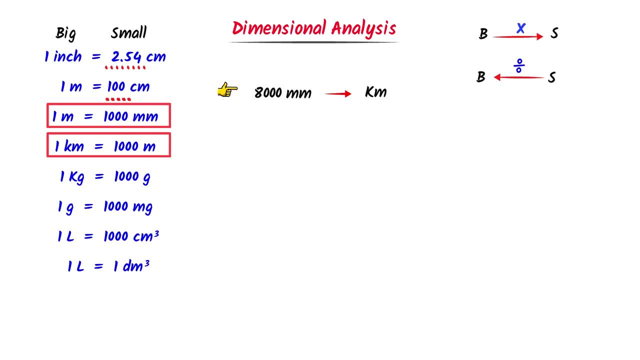 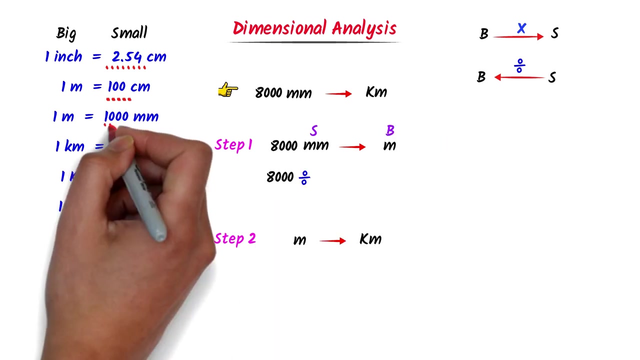 meter and kilometer. Hence I will solve this question in two steps. Firstly, I will convert millimeter to meter. Secondly, I will convert meter to kilometer. Now I write 8000 meter Here. millimeter is smaller unit and meter is bigger unit. I divide it by the conversion. 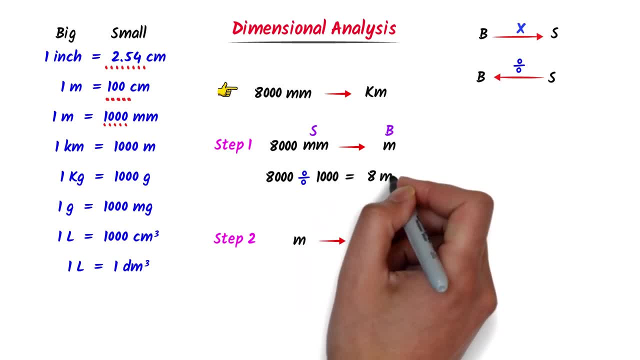 factor, which is 1000.. I get 8 meter. Now I will convert 8 meter to kilometer. Here meter is smaller unit and kilometer is bigger unit. I divide it by the conversion factor, which is 1000.. After: 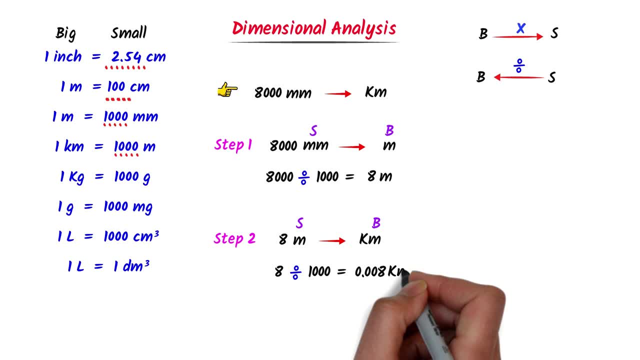 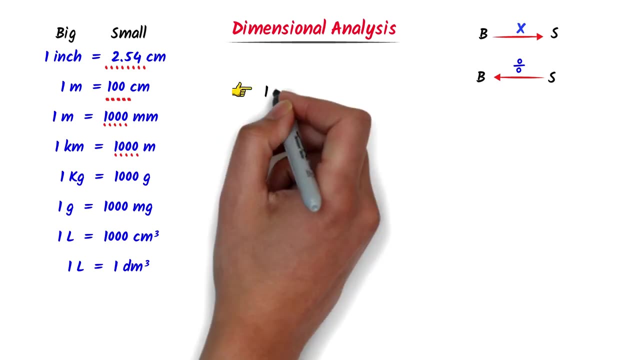 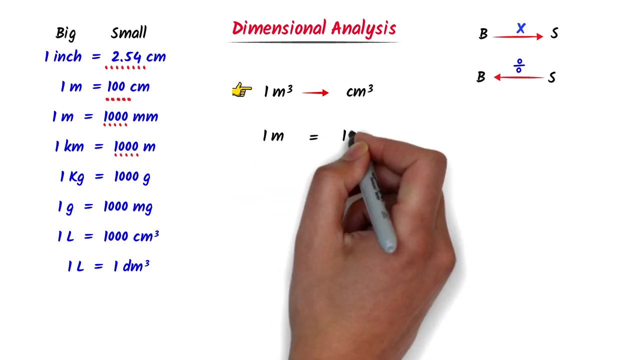 calculation, I get 0.008 kilometer. Thus 8000 millimeter is equal to 0.008 kilometer. Now let me teach you some hard level questions. Convert 1 meter cube to centimeter cube. Well, we already know that 1 meter is equal to 100 centimeter. Now the simple and easy trick. 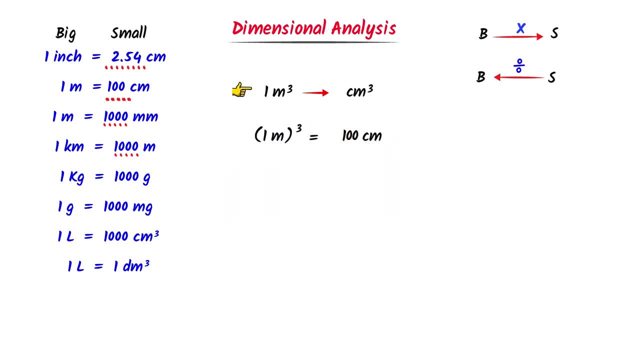 which I personally use is taking cube on both the sides. At the left hand side, cube on 1 is equal to 1.. Cube on meter is equal to meter cube, While at the right hand side cube on 100 means I write. 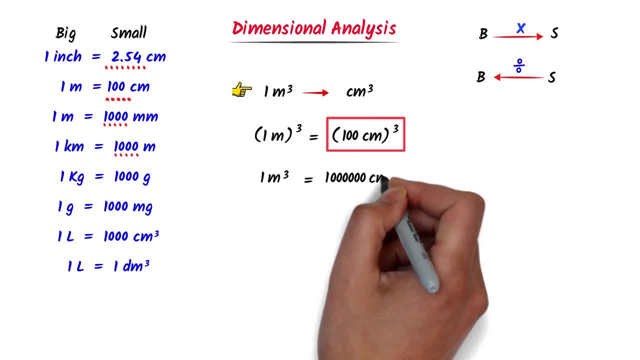 0.. This 3 on centimeter is equal to centimeter cube. Thus 1 meter cube is equal to 1 million centimeter cube, or 1 meter cube is equal to 10 to the power 6 centimeter cube. I write this relationship here. 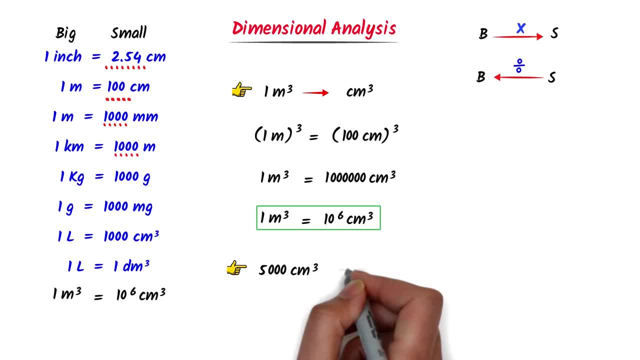 Now consider this question: Convert 5000 centimeter cube to meter cube. Well, I write 5000. Here meter cube is a smaller unit and meter cube is a bigger unit. I divide it by the conversion factor, which is 10 to the power 6.. After calculation I get 0.005 meter cube. Thus 5000 cm cube is equal. 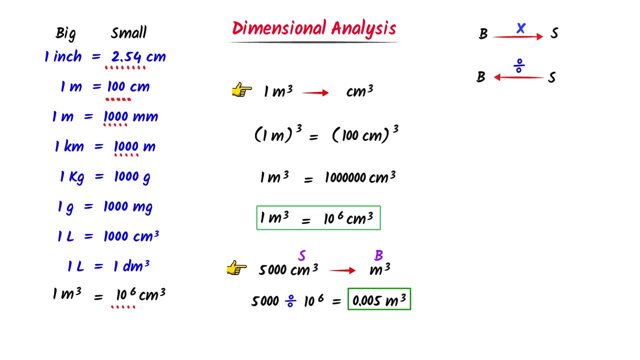 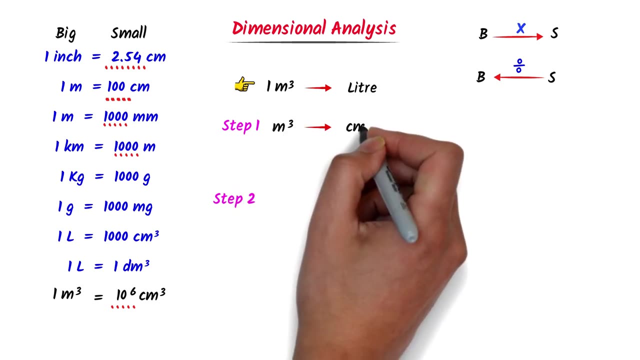 to 0.005 meter cube. Lastly, let me teach you one bonus question: Convert 1 meter cube to centimeter cube. Well, I will solve it in two steps. Firstly, I will convert meter cube to centimeter cube. Secondly, I will convert centimeter cube to liter. Now we already know that 1 meter cube is: 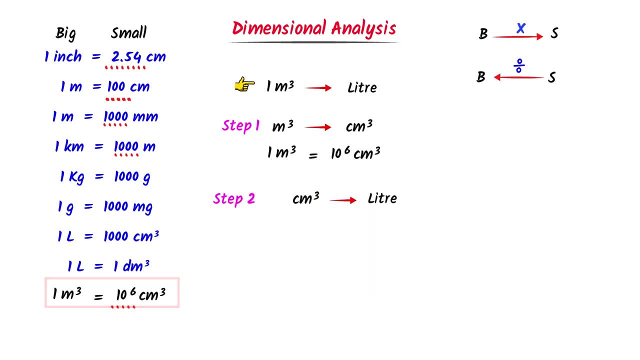 equal to 10 to the power 6 centimeter cube. So I converted meter cube to centimeter cube. Secondly, I take this 10 to the power 6 centimeter cube and I write it here Now. according to this relationship, centimeter cube is a smaller unit and liter is a bigger unit. 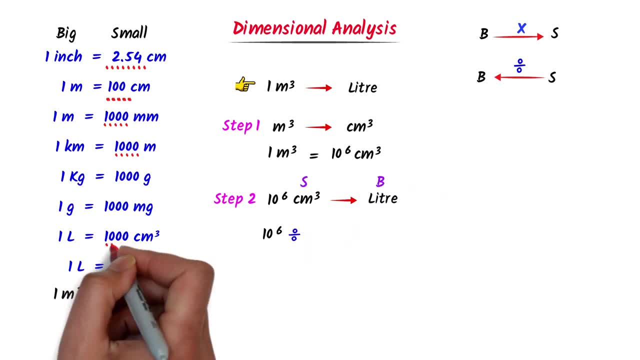 So I divide this 10 to the power 6 by the conversion factor, which is 1000.. After calculation I get 1000 liters. Thus 1 meter cube is equal to 1000 liters. I write this relationship here: 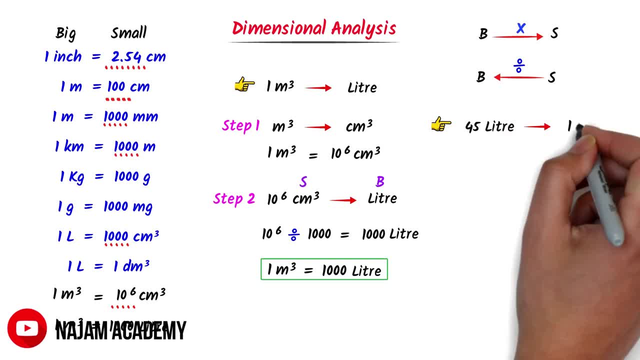 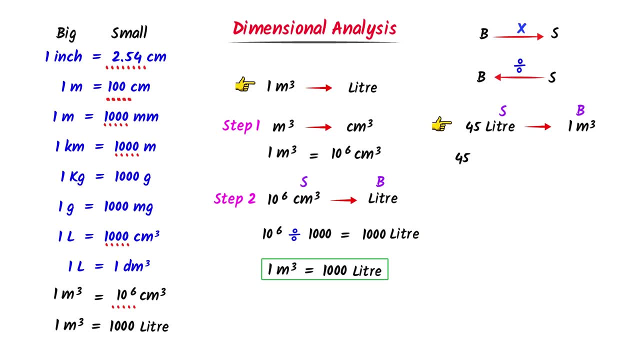 Lastly, I convert 45 liters to meters cube. Lastly, convert 45 liters to meters cube, So cube. well, I write here 45. we know that liter is a smaller unit and meter cube is a bigger unit. I divide 45 by the conversion factor, which is thousand. 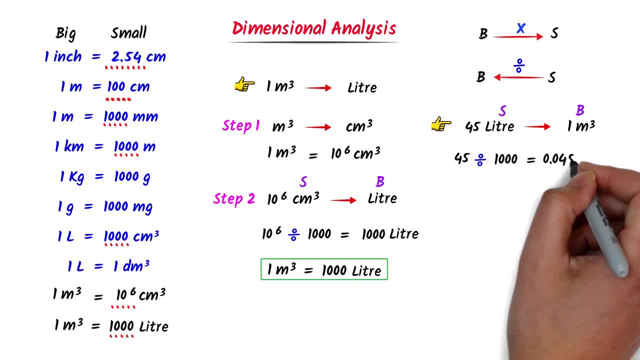 after calculation, I get 0.045 meter cube. thus, 45 liter is equal to 0.045 meter cube. therefore, using this trick, we can easily learn dimensional analysis. I hope that you have learned all these important concepts.